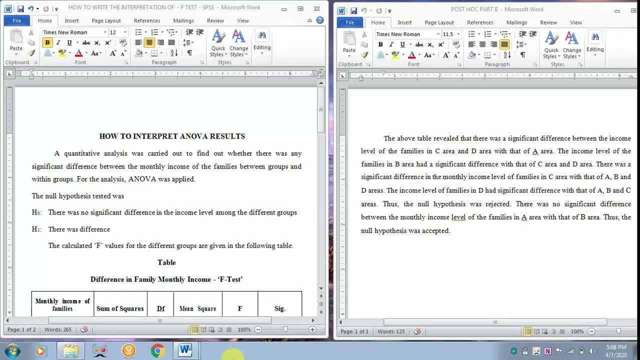 Today I will be teaching as to how to interpret ANOVA results. Here you can see I have taken the family monthly income where I have got four groups. When you are doing ANOVA you should have more than two groups. So a small intro with its hypothesis is given on the 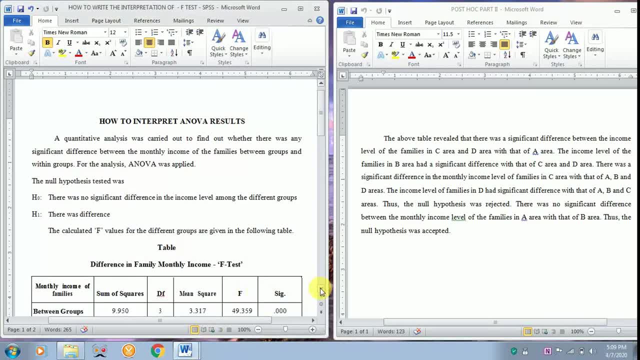 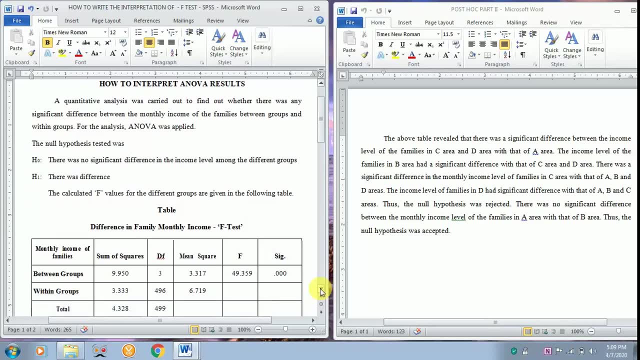 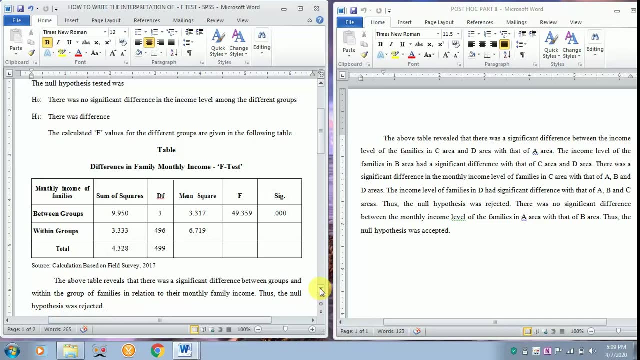 screen. Quantitative analysis was carried out to find whether there is any significant difference in the monthly income. The next is in the null hypothesis and the next is the f value. The f value should be significant to show that the model is fit. So after writing. 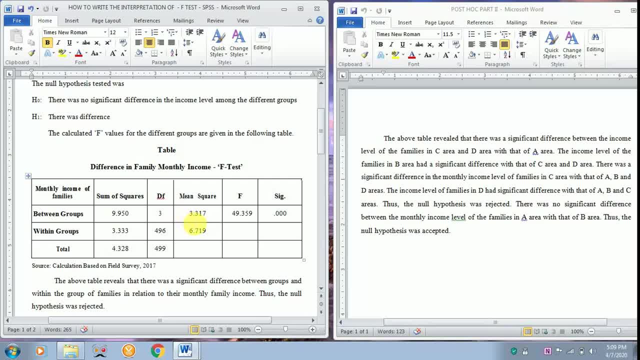 the values in the respective column You have two groups have to explain that. the above table reveals that there was a significant difference between groups and within groups of families in relation to their family income. thus the null hypothesis was rejected. now later we are going to post hoc test for that. i am just scrolling down. 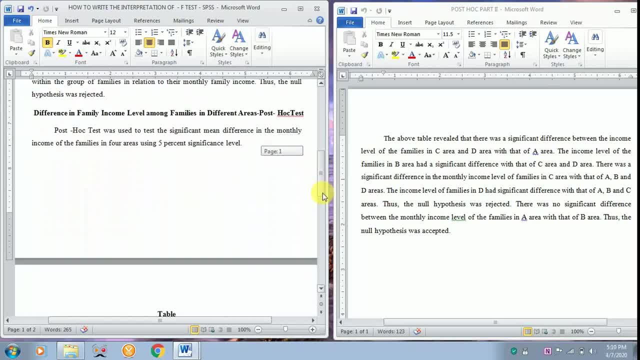 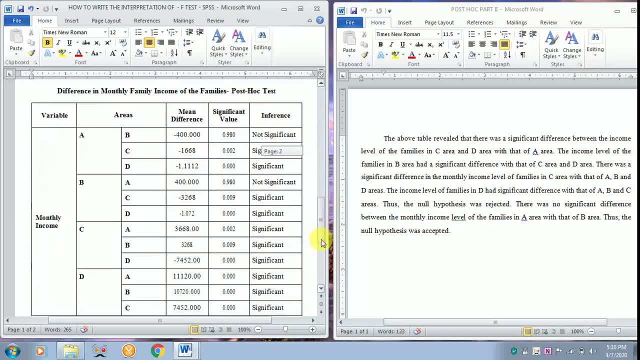 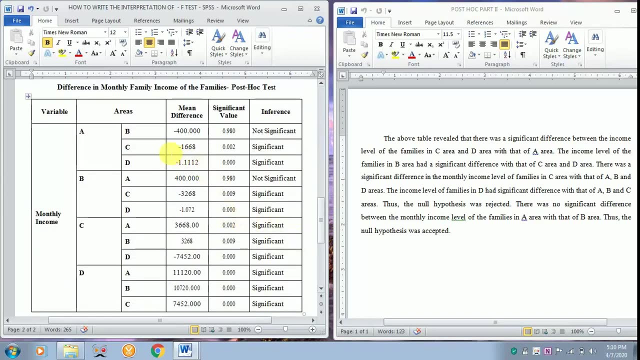 so post hoc is done to find out whether there is a difference in the income earned by the people in the four areas. so you can see these are the areas a, with that of b, c, d and mean difference, the significant value and the inference of it. this is otherwise called the. 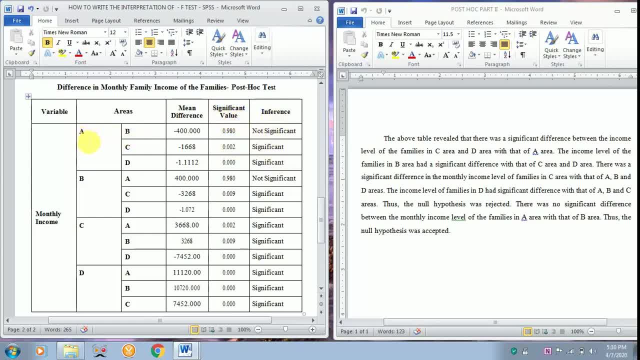 as p value. so you can find that in the case of a and b it is not significant, but that of a and c it is significant, and a and d also is significant. so when i say it is significant, you have to check up with your average mean and find out who is earning more, whether a area or c area or a or d. 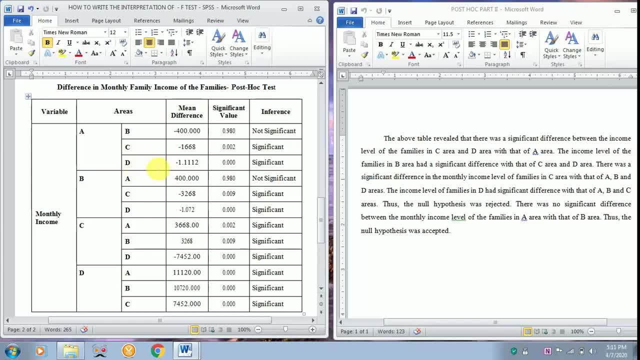 and later interpret in your results. similarly, in the case of b, b and c, and b and d are significant because the p value is less than 0.05. the case of c- all the three, there is a significant difference. d also, there is a significant difference on the right hand side. you can see the interpretation.